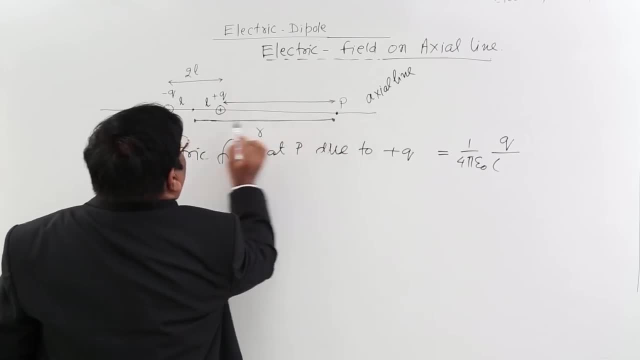 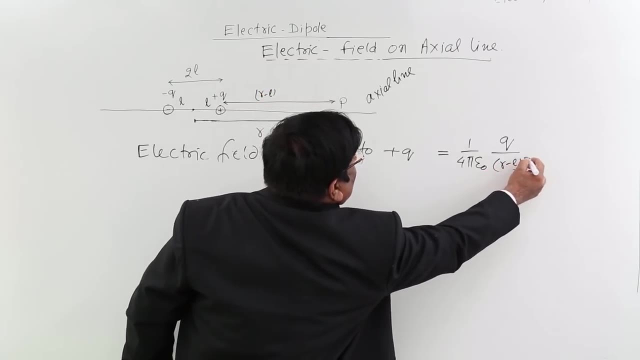 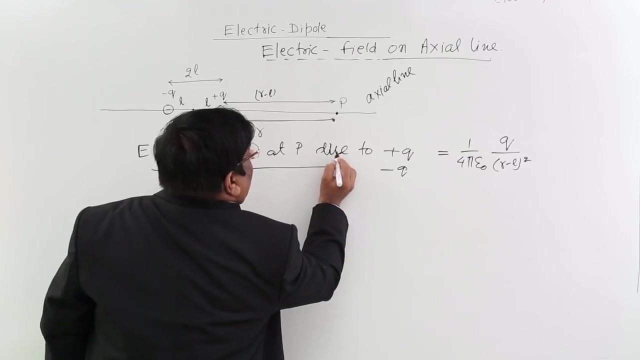 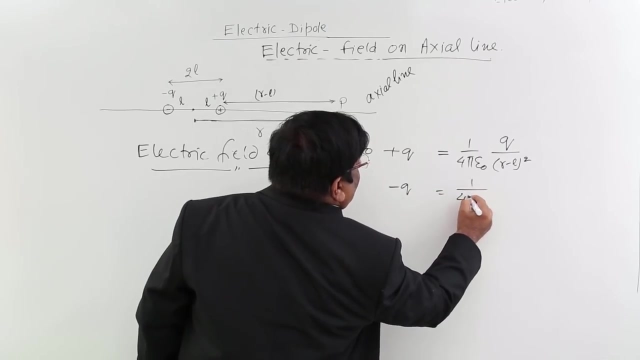 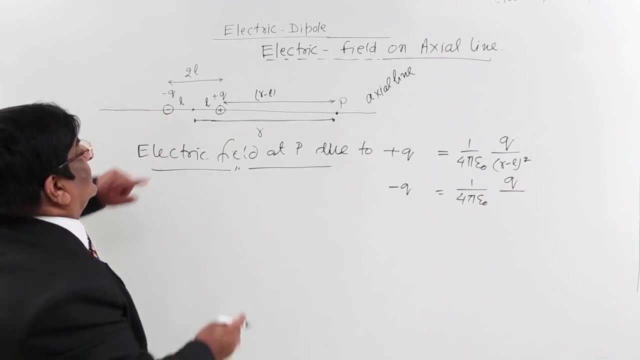 make. if this is, if this distance is r, this distance is L, then this is r minus L and this will be r minus L square. Similarly, electric field at P, due to minus Q. Due to minus Q, this we can make as 1 upon 4 pi, epsilon 0 Q upon this distance. This distance is r plus. 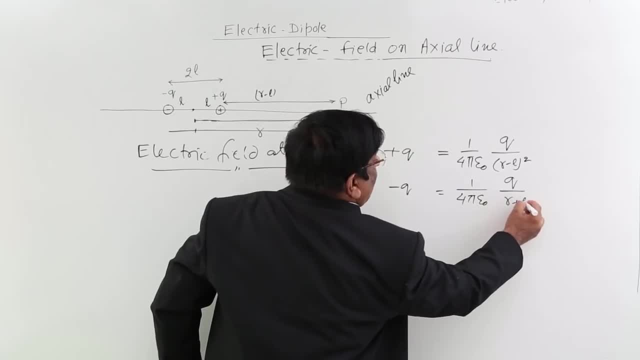 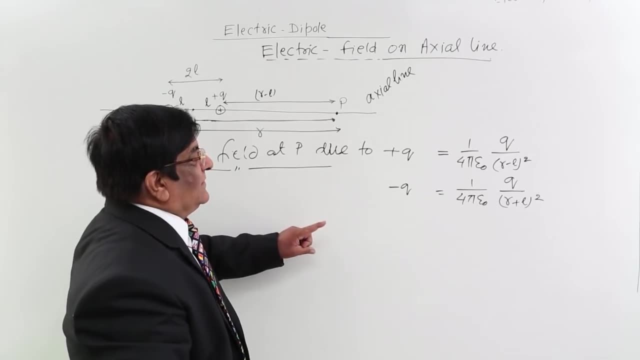 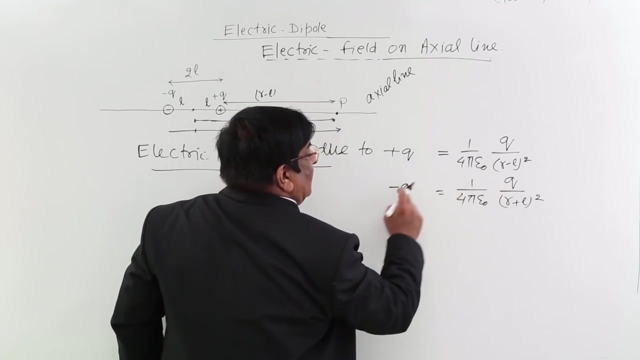 L. So this is r plus L and this is r minus L. So this is r plus L and this is 2 pi epsilon L square. Now there are two methods. if you want, you can keep the electric field along with sign this is because of the negative Q. then this E will be negative minus and this 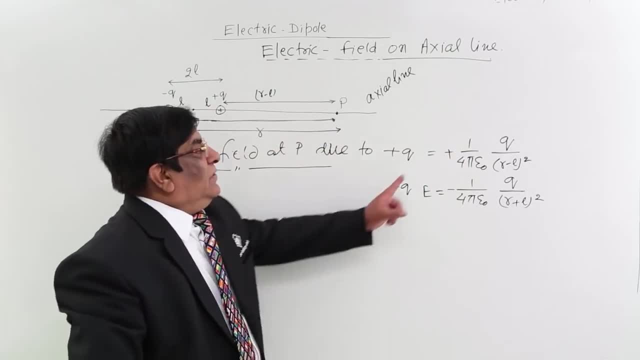 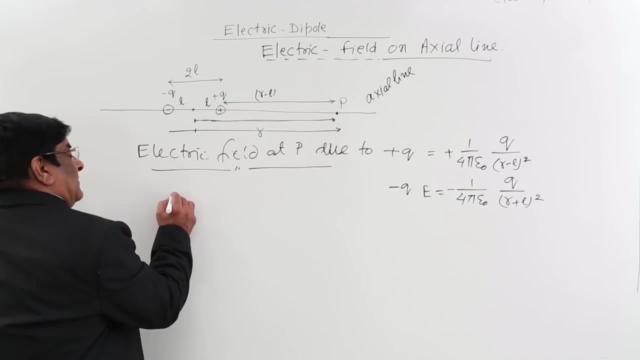 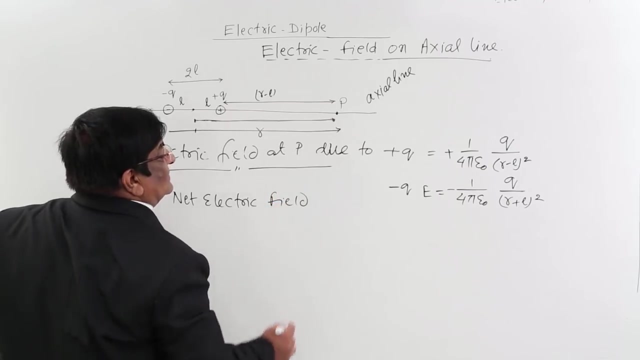 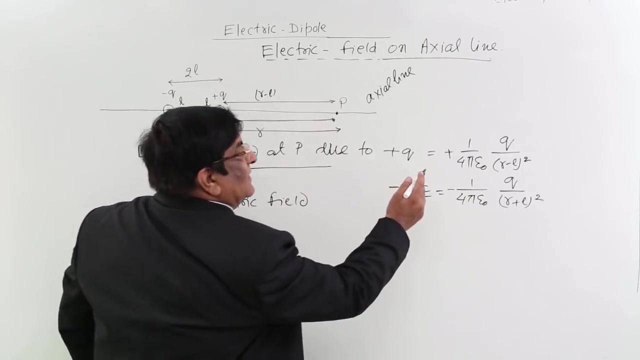 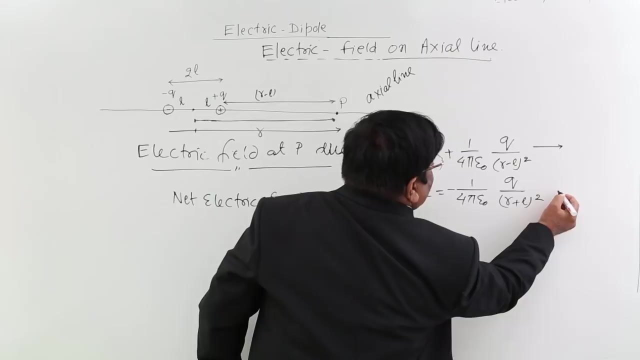 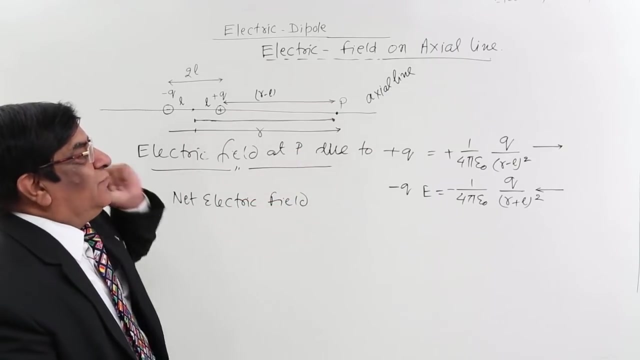 will be positive. So we can make it like this, or when we are finding the electric field. net electric field is addition of the two. Electric field is a vector quantity. this is positive electric field. its direction is this way. that is positive direction. This is negative. its direction is this way. Now, if we want resultant, then what do we do? 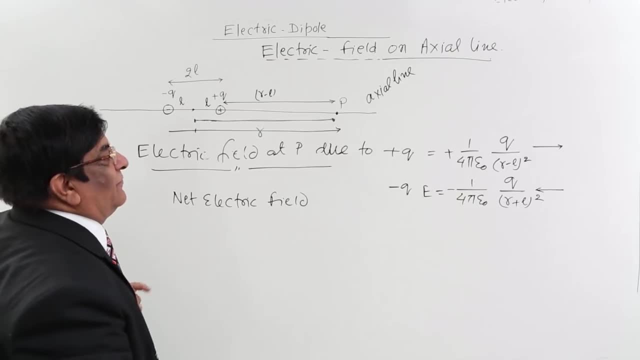 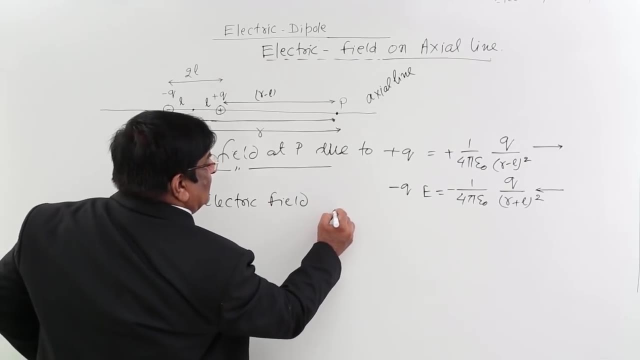 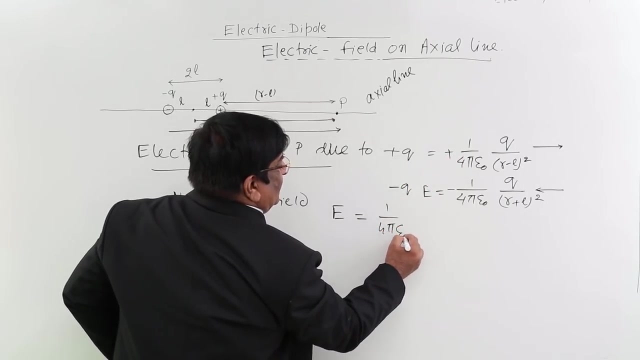 according to our training in the vector addition, we know that we must decrease one from the other because they are in opposite direction. So net electric field E net will be 1 upon 4 pi epsilon naught, which is the larger one whose denomination is negative. 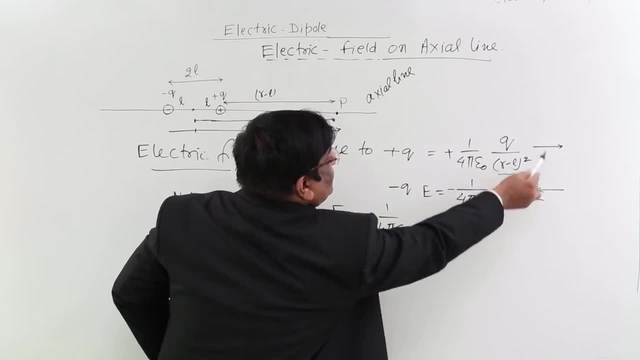 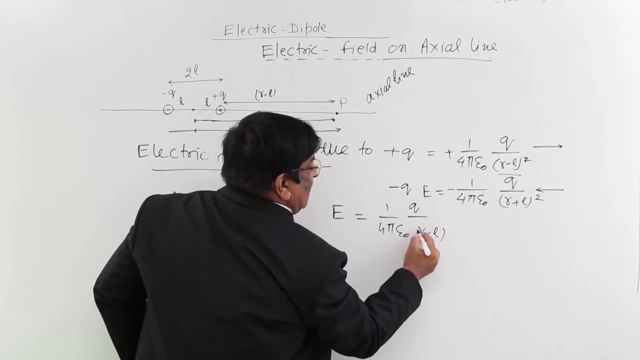 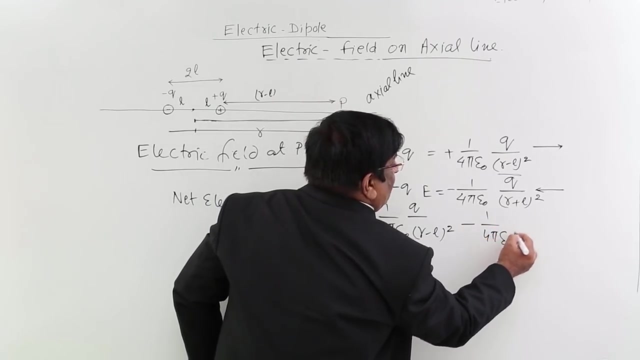 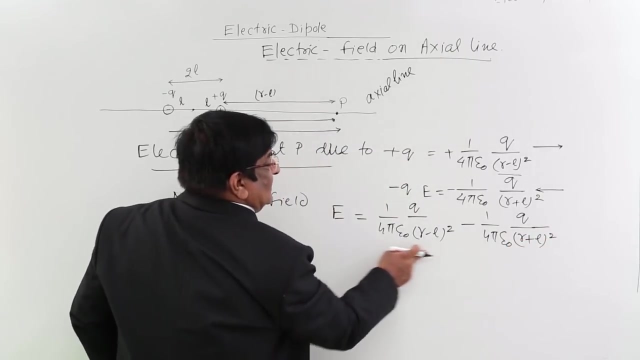 This denomination is smaller, so this field is larger. this will prevail. how much will be the net? Q upon R minus L square and minus 1 upon 4 pi. epsilon naught Q upon R plus L square. this is in this direction. this is in this direction, so this will be net. And now, 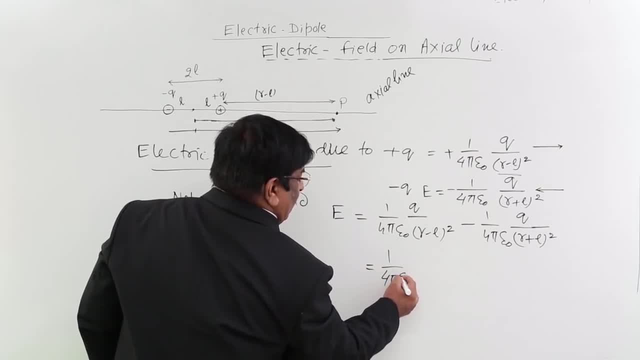 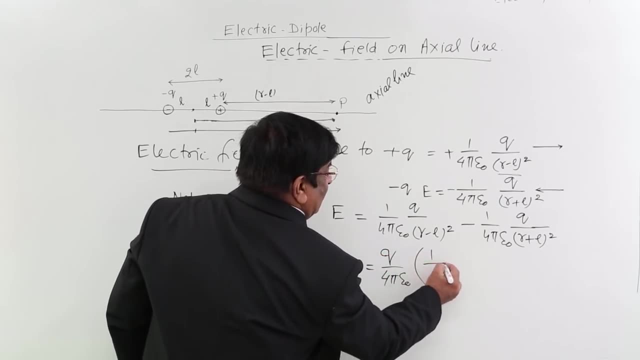 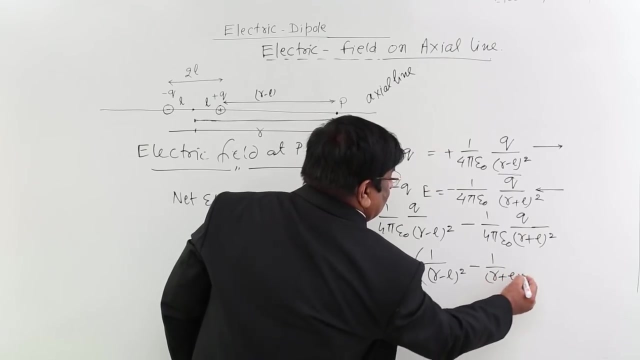 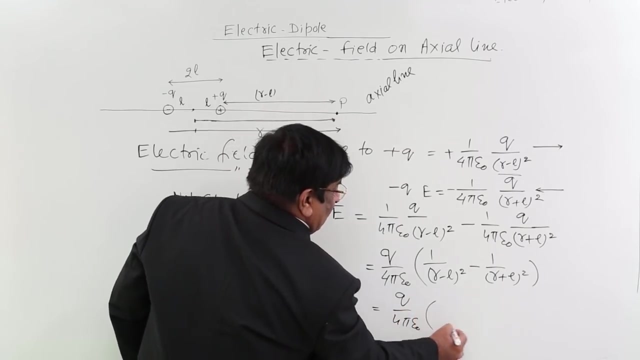 we have to calculate the net Q upon R minus L square, minus 1 upon R plus L square. This is common. Q is also common, and what we get inside is 1 upon R minus L square, minus 1 upon R plus L square. this is Q upon 4, pi, epsilon naught, and here we get: multiply the. 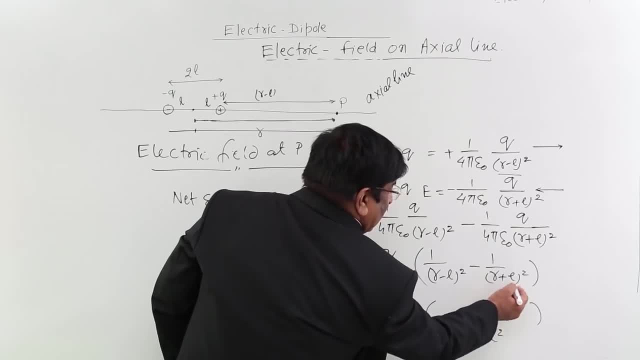 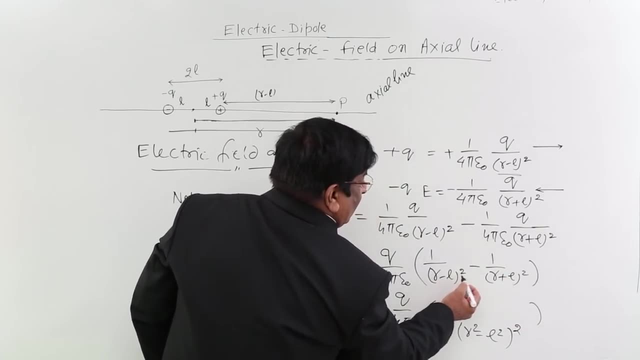 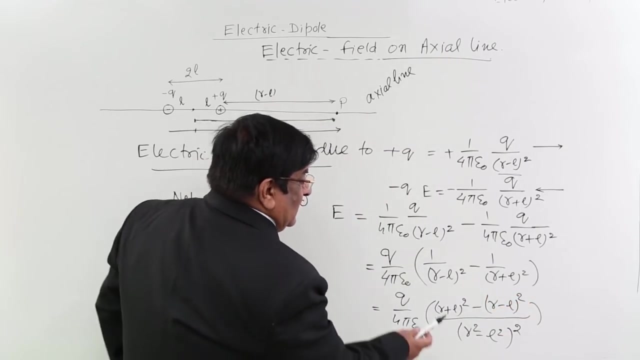 two R square minus L square. This square is here inside. we have multiplied R square minus L square. this and here, if we divide with this, what remains R plus L square minus. divide with this, what is remaining is R minus L whole square. If you solve this, 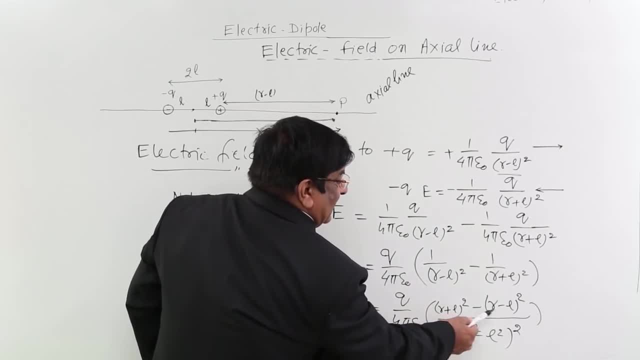 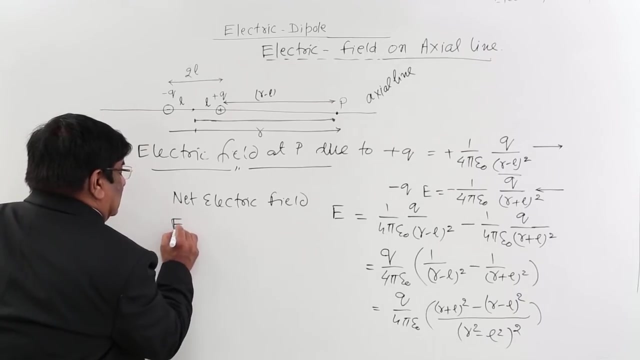 Now, if we take the L square and minus R square, L square minus L square, cancel out what we get here: 2 R L minus minus 2 R L. that will added up to 4 R L. So now I come here. the net electric field E. E is equal to Q upon 4 pi. epsilon naught. 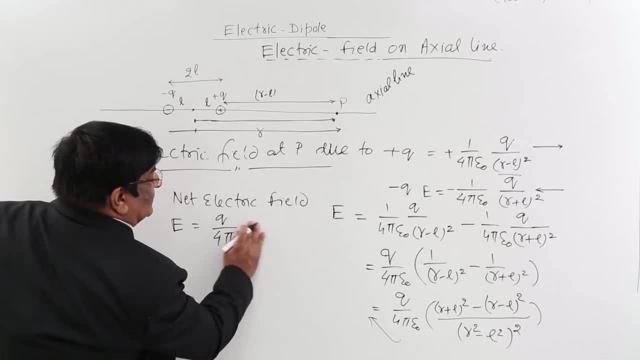 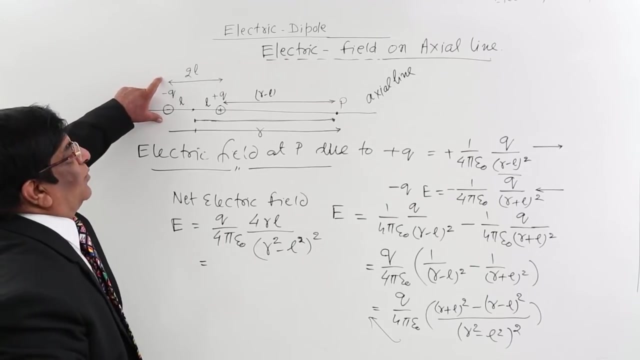 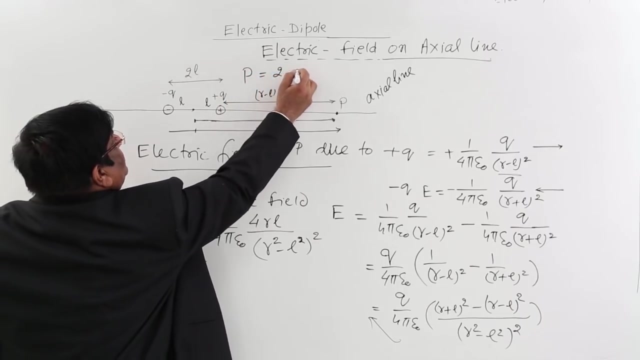 and this will be 2 and 2.. 2, 4 R L upon R square minus L square, whole square. Now we know a quantity, that is dipole moment, effectiveness of the dipole, and that dipole moment. we know the formula. it is 2 Q L Here. 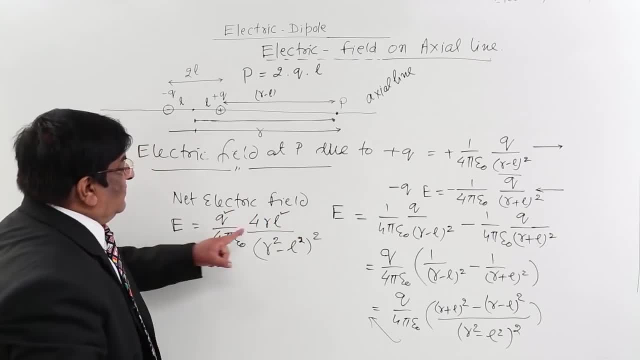 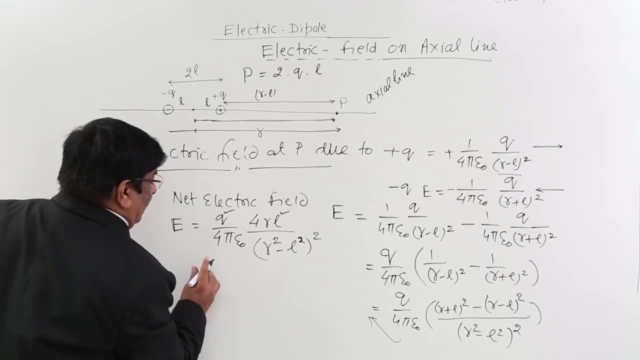 we take this: Q is here, L is here, and 1, 2 we will take from here. So what we can write in place of 2, Q, L, we will write P, So that is P. What remains here is 2 R upon 4 pi, epsilon. 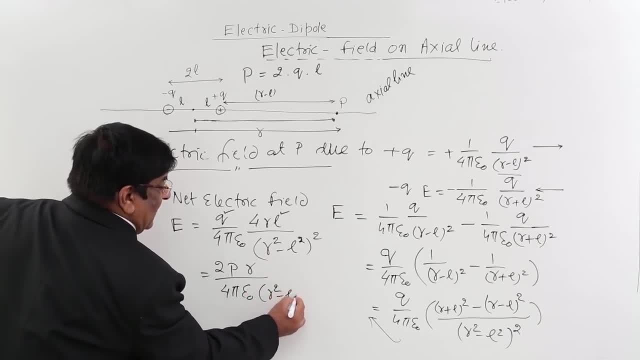 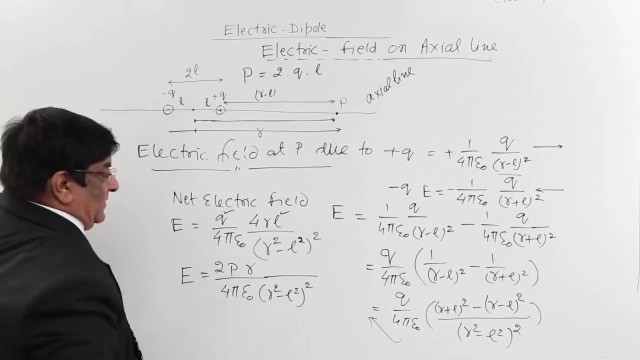 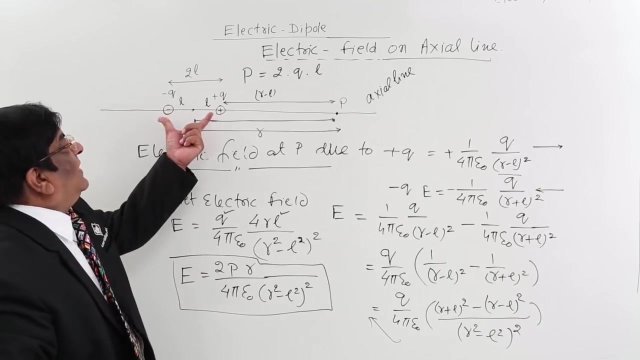 naught, and this is R square minus L square to the power 2.. This is actual electric field. But here we can make certain approximations. The approximation is, the dipoles are very small in size, So L is very small. Compared to any distance of R, L is very, very small. 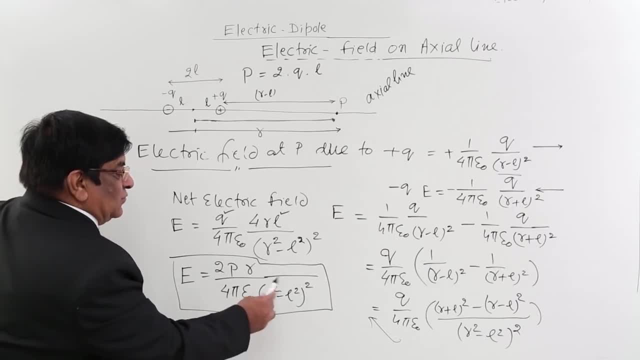 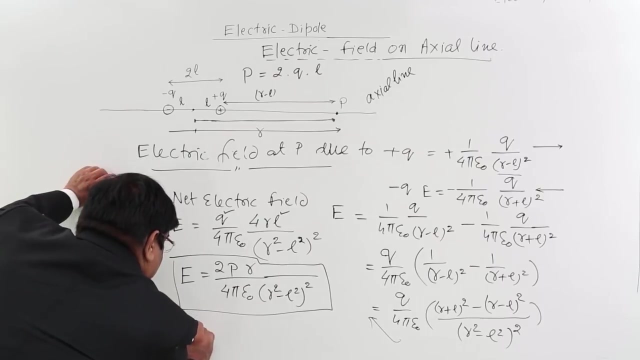 quantity. So when it comes to minus or plus, square of R decreased by square of L does not make any significance change in R square value. So this L square we can write Right: OMIT. So L square is very small. L square very small compared to R square, Hence neglect. 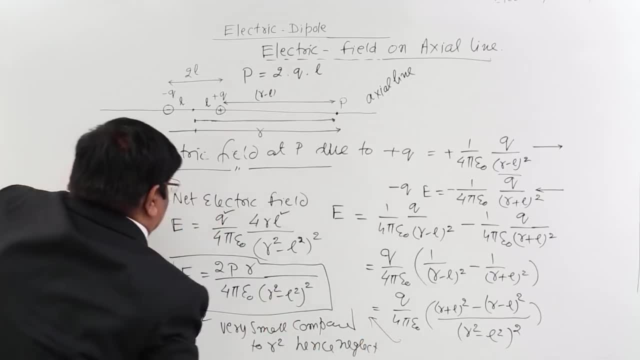 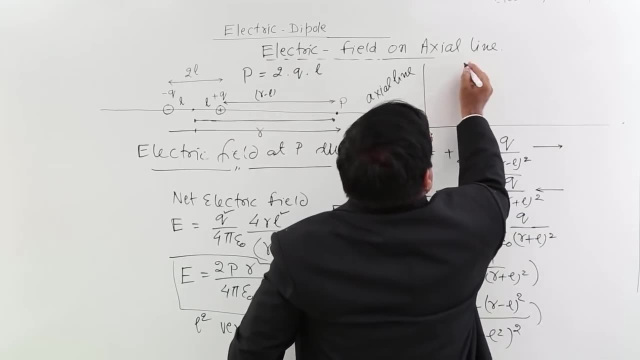 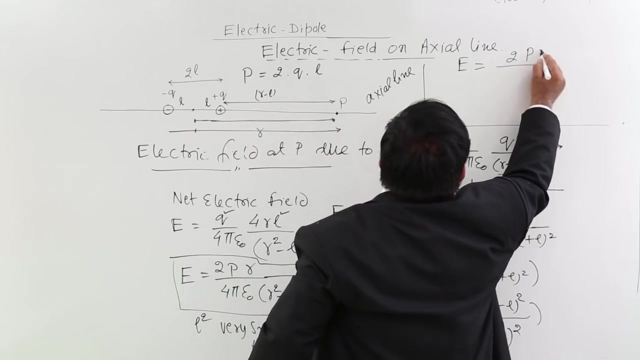 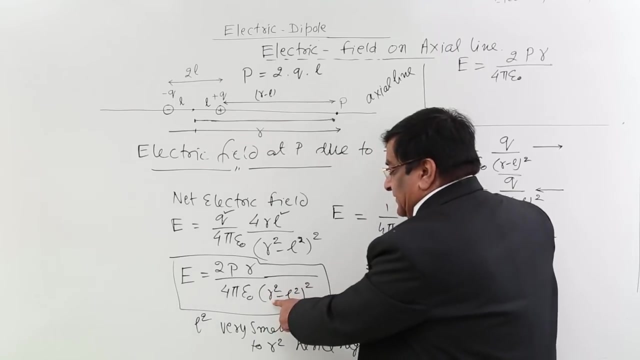 it. And now, if we neglect it, what remains with us? that I will write here: E? E is only the deleته equal to 2 p? r divided by 4 pi, epsilon 0, and this is r square square. r square square is: 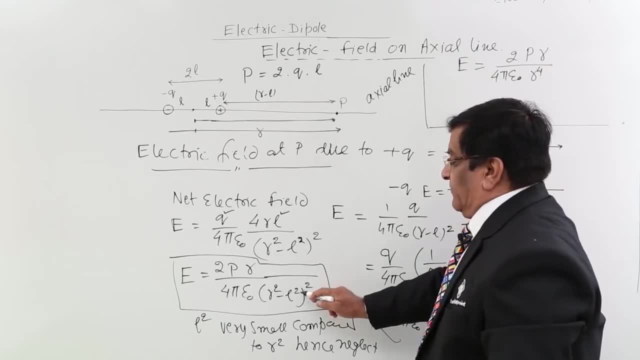 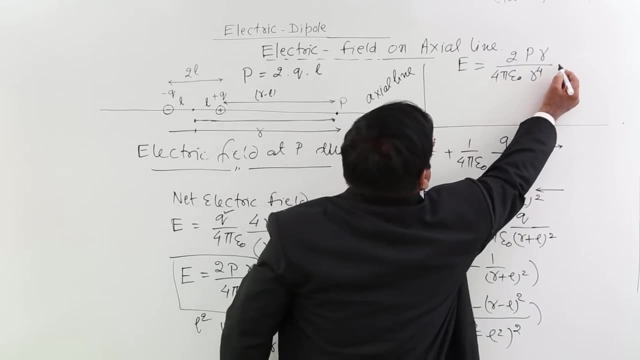 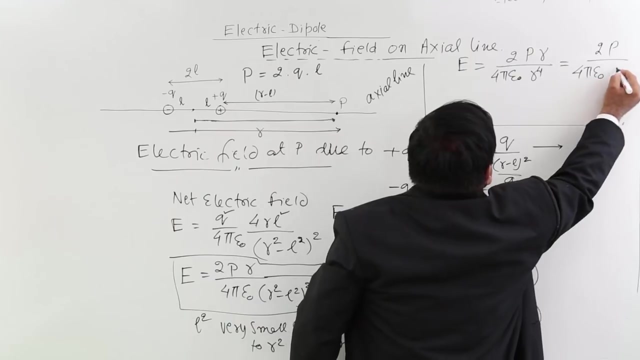 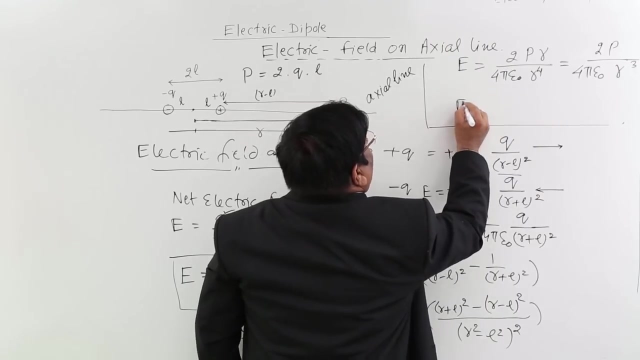 r to the power 4 and l. we have neglected. this is our expression. Now, if this is our expression, then r, r can be cancelled and what we get here is 2 p upon 4 pi, epsilon 0 r to the power 3.. This is the simplest one we can get and we can write it. 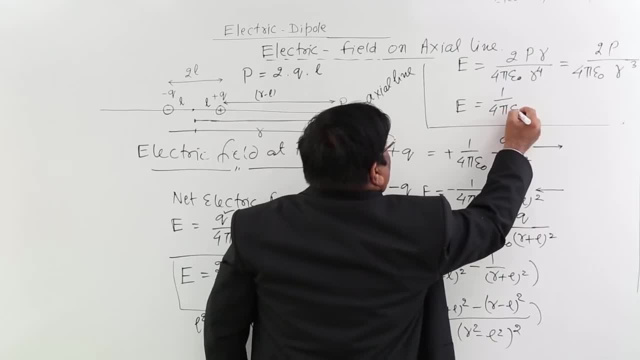 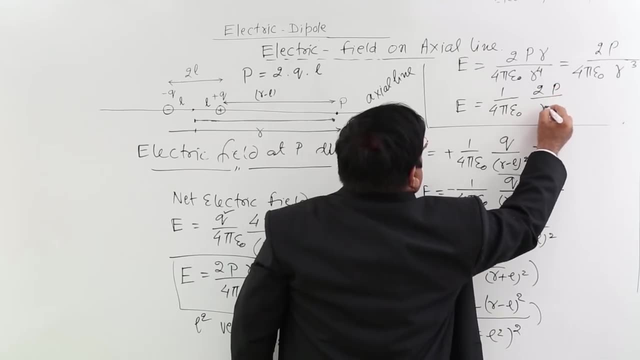 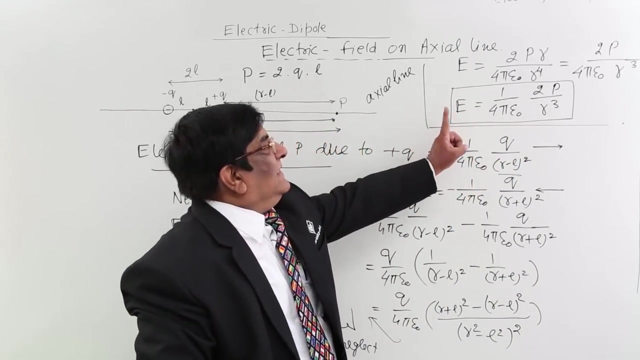 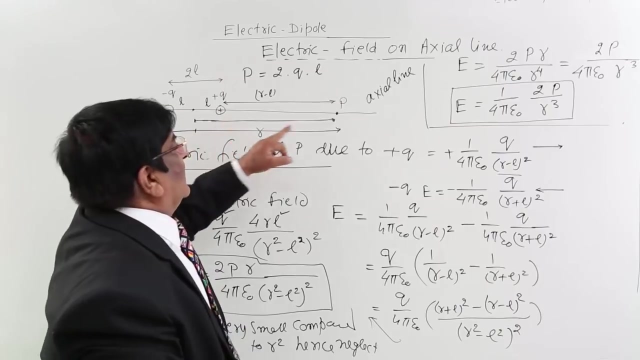 this way, e is equal to 1 upon 4 pi, epsilon 0, which is constant, of the medium, and here we have 2 p upon r cube. So this is our result, which we will remember: that electric field is not 0. It has certain value. So this we have seen on the excel line, it has certain value. Now, 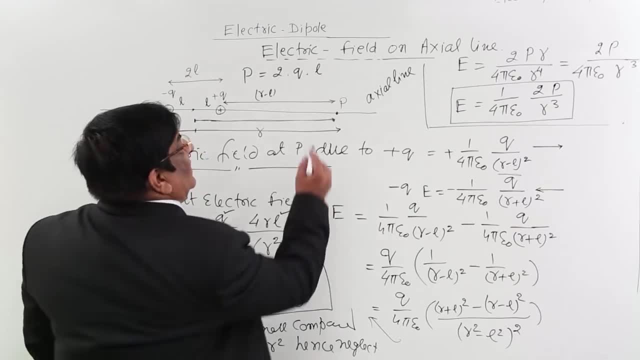 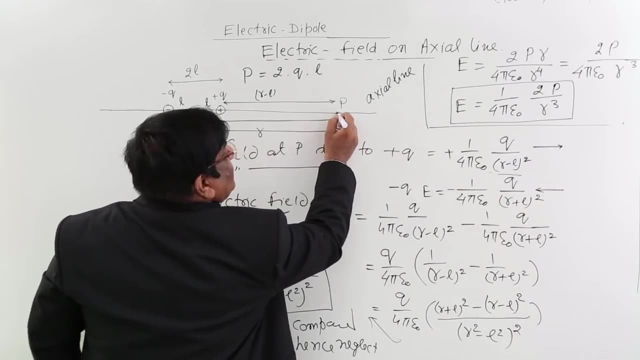 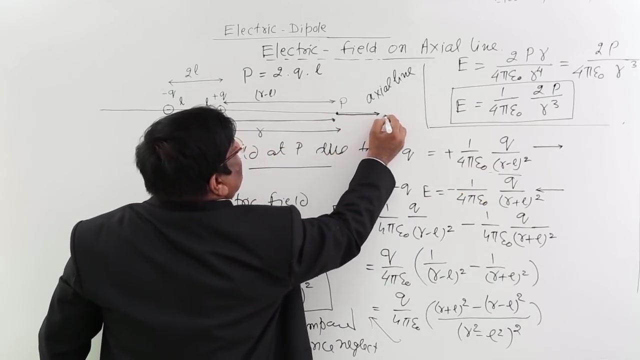 this is magnitude of the electric field. What should be the direction? Answer is that we have done earlier. this is a larger quantity and it has got direction this way and this is smaller, cancelled out. So what we get remainder is electric field in this direction. 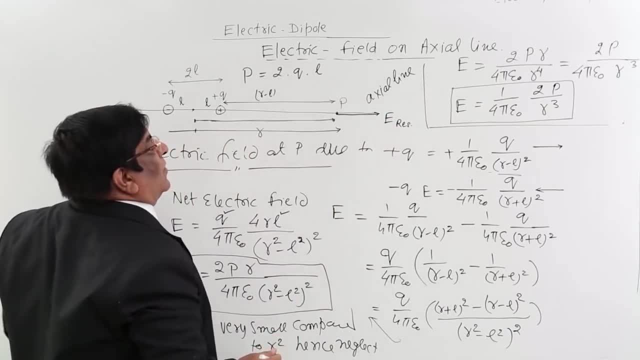 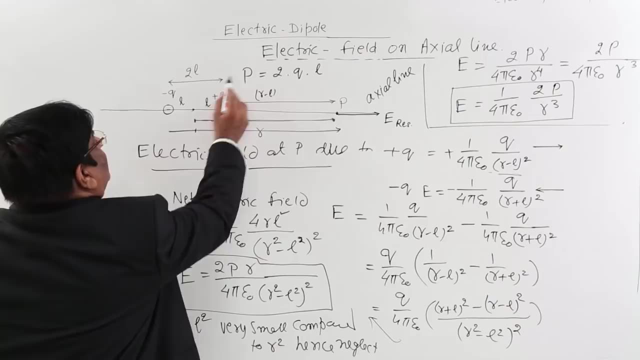 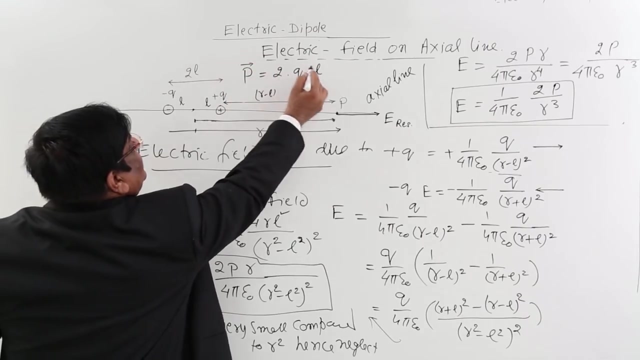 This is our resultant electric field. Now, how do we know that electric field is not 0.. How do we name this direction For nomenclature? see this, dipole moment is a vector quantity and it has got a particular direction. What is the direction of dipole moment Minus to? 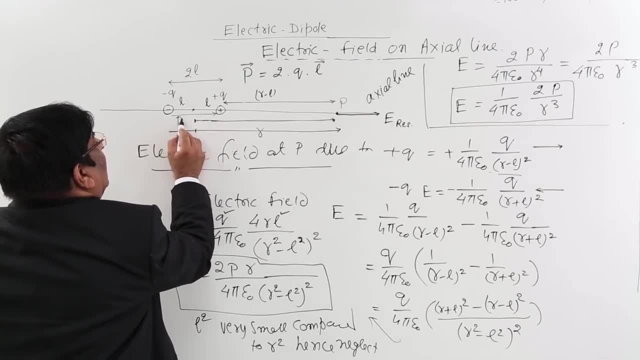 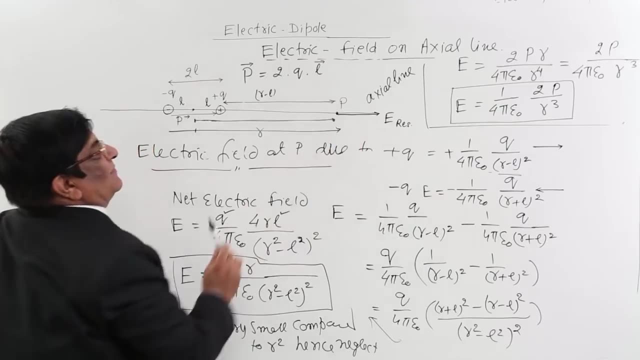 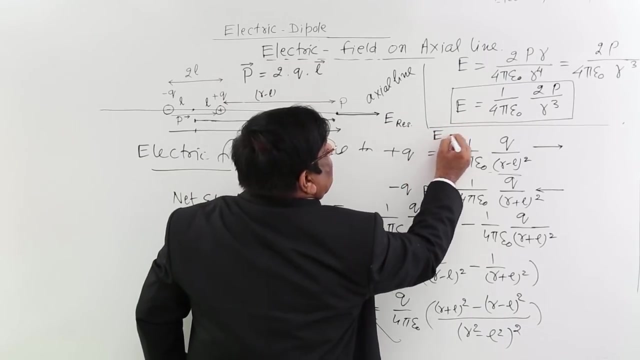 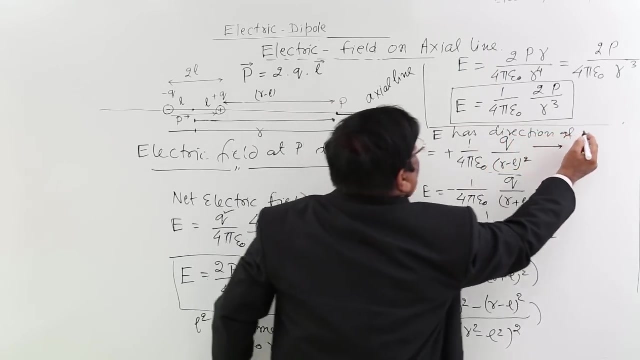 plus. So this is direction of dipole moment. We will compare with this electric field and dipole moment. Both are in the same direction. So this is the direction and this is how we remember it, That E has. E has direction of dipole moment, dipole moment. 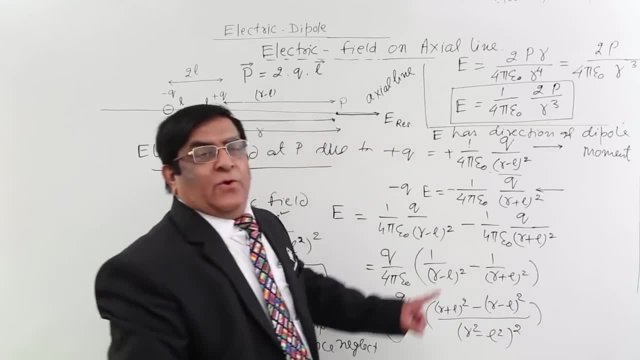 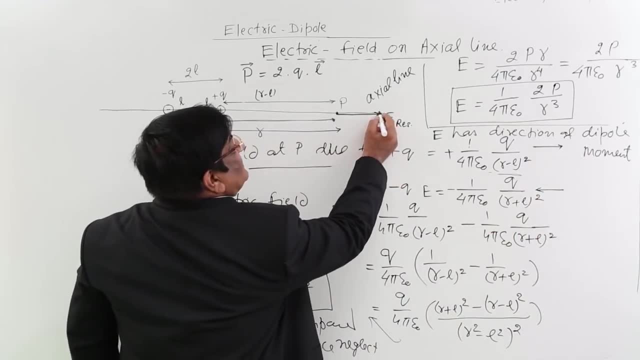 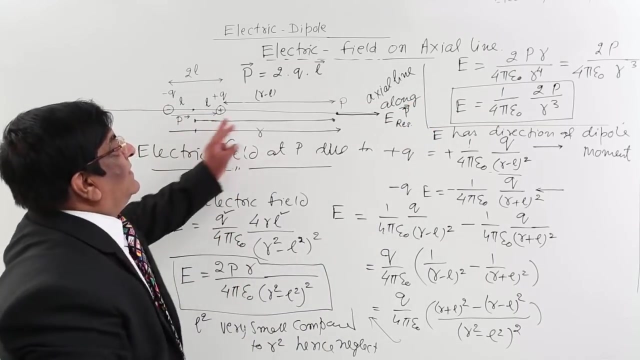 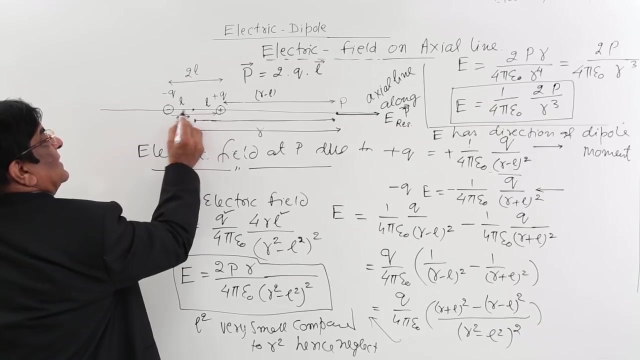 Okay, so now we get: this is magnitude and this is direction. We will say: this is another word for this is along p. along p means whatever is the direction of p. that is direction of E here. if you will take it here, it is in this direction. if you will take it here, it is in this direction. 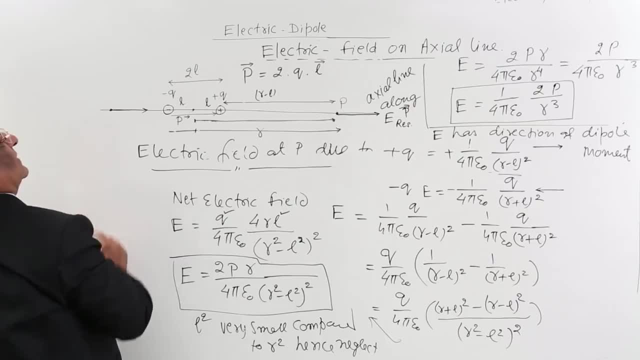 if you will take it here again, it is in this direction. don't think that it will revert. it will not. you see, minus will attract a test charge in this direction, plus will repel it in this direction. but this is away. so here this force will be prominent, this force will. 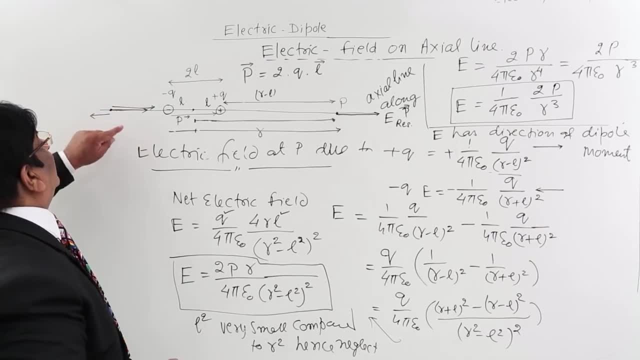 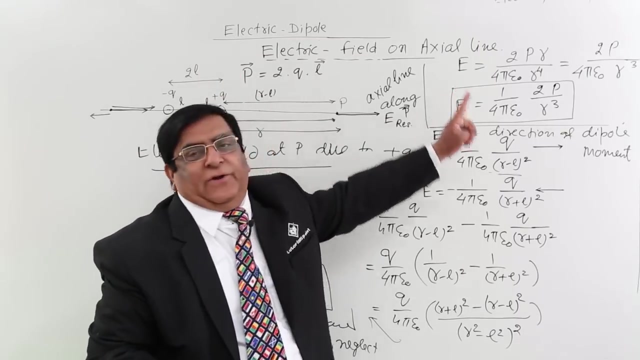 be larger, this electric field will be larger. so net electric field will be again in this direction, so completely on the x line. at any point electric field is always in the direction of p and this is the formula for that. so next we will study what will be the electric field. due to dipole on the transversal line. 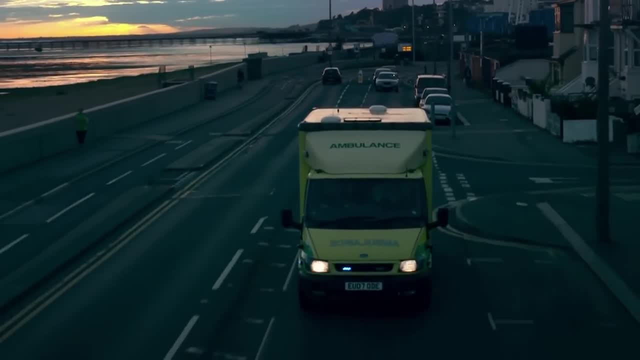 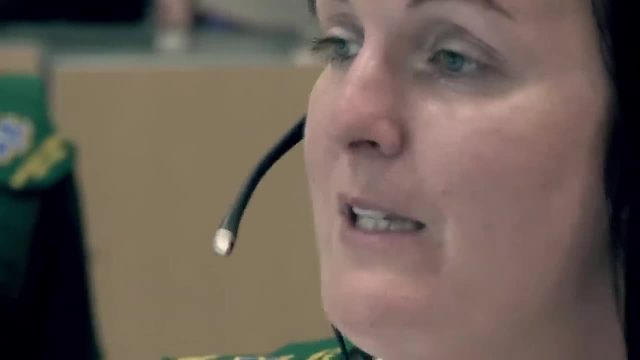 Another day breaks Short sigh. For some it will be the best day of their life. for others it will be the worst. I'm going to have to tell me exactly what's happened. There's one emergency service that gets to know us more intimately than any other. 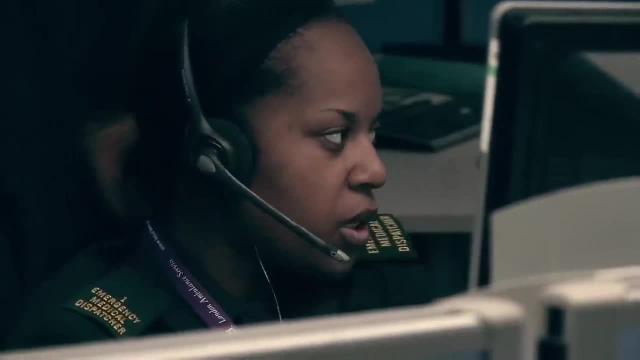 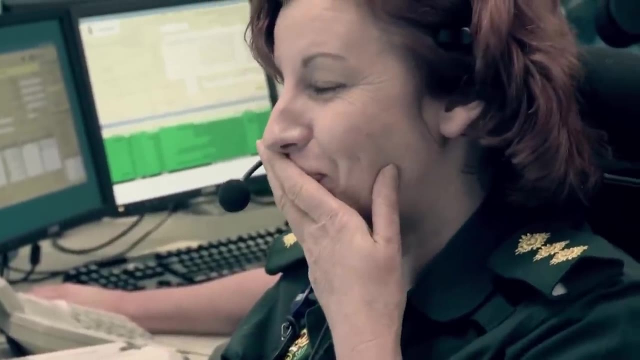 If you feel sick and you need to vomit, just vomit, but let me know when you're finished. When you called in, you said that she'd been drinking and she'd messed herself. They'll spill everything out to us. For some reason, they seem to think we hold all the answers.